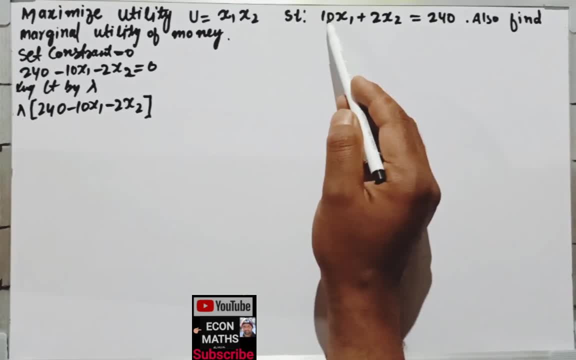 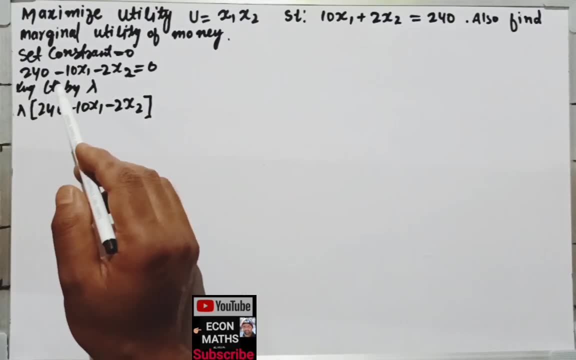 this will become 240 and we will transpose this. This will become minus 10x and minus 2x2.. That I have written here. After that we will multiply this constraint by lambda. Now the third step is: we will form the Lagrange's function Now. 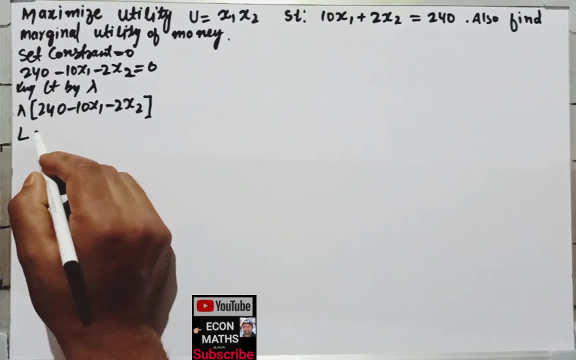 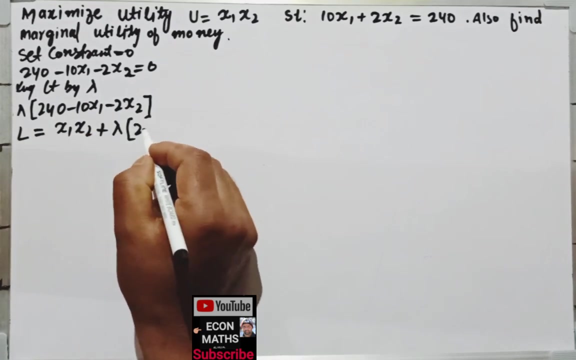 lagrange's function is formed by. lagrange's function is formed by: adding the objective function with the with this uh constraint, so this will become x1, x2 plus adding this constraint after multiplying it by lambda, so this will become lambda times 240 minus 10 x1. 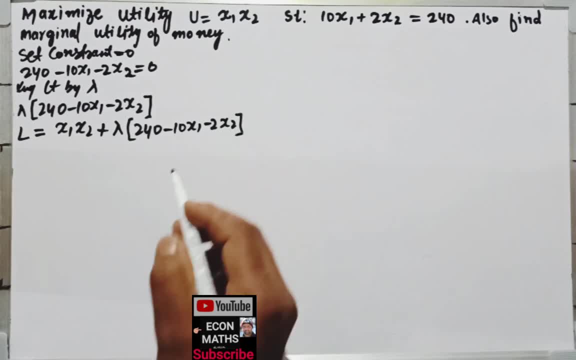 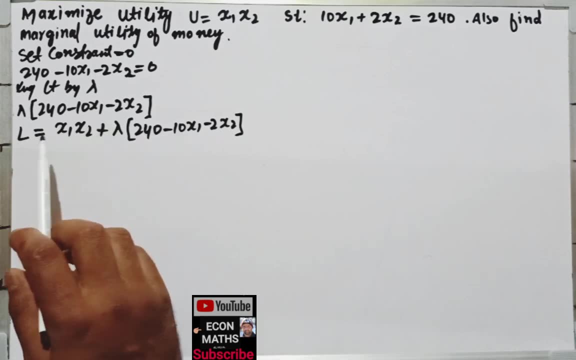 minus 2, x2. now this is our lagrange's function now to get the optimal values of x1 and x2. we will partially differentiate this lagrange's function with respect to x1, x2 and lambda and set them equal to 0. so we will partially differentiate this, partially differentiating. 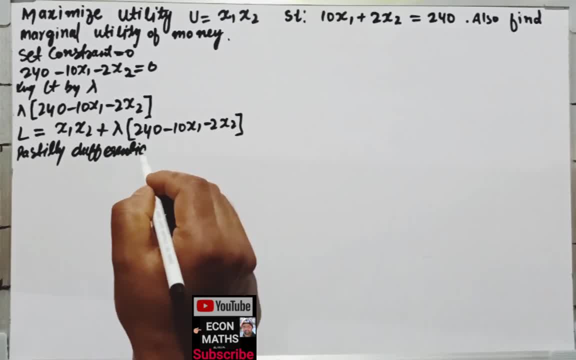 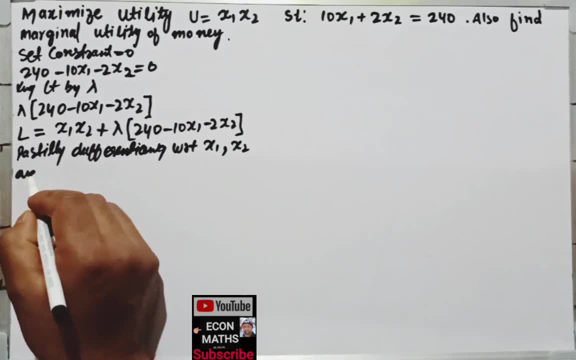 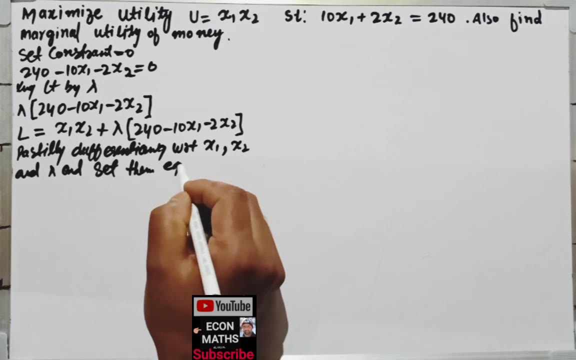 x1, x2 and lambda and set them equal to 0. so we will partially differentiate this, differentiating with respect to x1, x2 and lambda and set them equal to them, equal to 0. so we will see. now i will write: l of 1 means i am differentiating this. 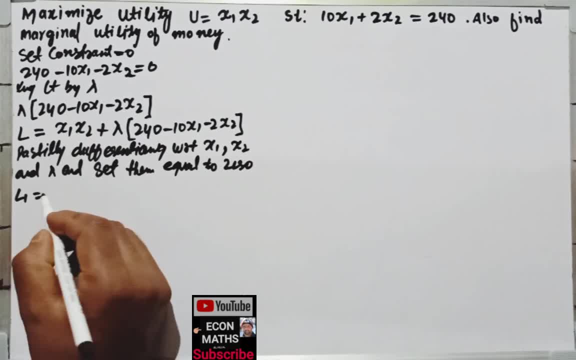 lagrange's function with respect to x1. now this will become here the. the derivative of x1 and x2 is the derivative of x1 and x2 is the derivative of x1 and x2 is 0. so here i got this x2, plus now lambda into 240, since no x1 is involved. so derivative is 0. 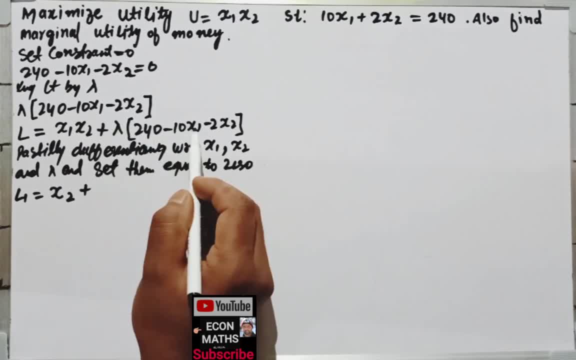 now lambda into minus 10 x1. so here this will become minus 10, because the derivative x1 is 1, so this will become 10 lambda and i will set it equal to 0 or i can write it as: x2 is equal to 10 lambda. now let this be equation first. similarly, we will differentiate. 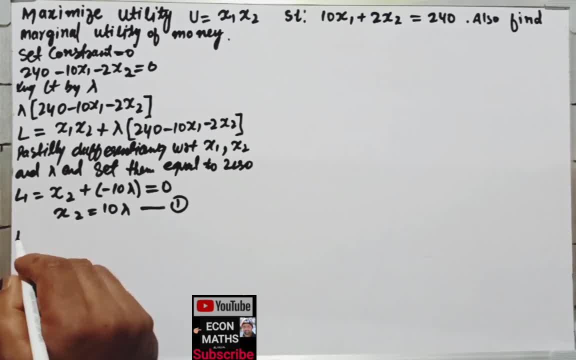 this with respect to x2. so l2 means differentiating this lagrange's function with respect to x2. now here it will become. the derivative of x2 is 1, so here we got x1, now here it is plus. so i will write here now lambda 240. no, x2 is invalid, so derivative is 0 because the derivative of constant. sorry. 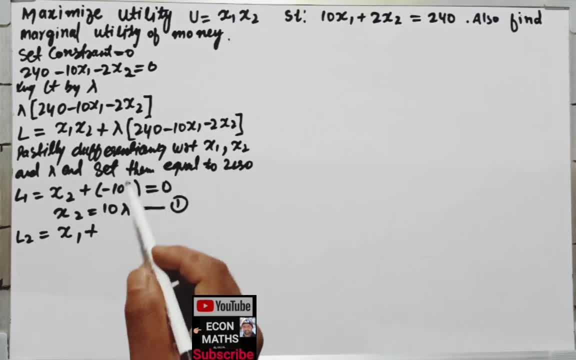 because no x2 invalid, so its derivative is 0. similarly, lambda into 10: x1: no x2 is invalid, so derivative is 0. now lambda into minus 2: x2. here the derivative of x2 is 1. now lambda into minus 2: will we get here? so this is minus 2 lambda, now set this. is this also equal to 0? 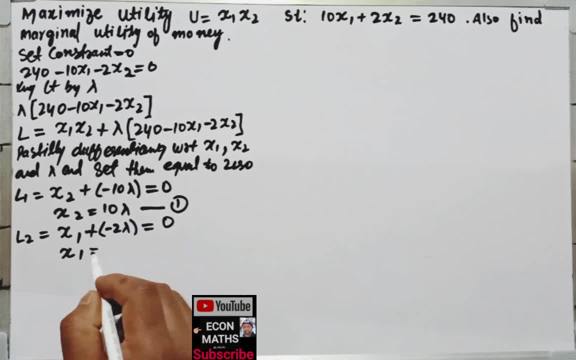 now further writing: this is x1 is equal to now. transposing this on our hs, this will become plus plus 2 lambda. now let this be equation. second, similarly differentiating this lag resist function with respect to lambda, so as of lambda is equal to now, since in this part no lambda is involved, so derivative is 0. 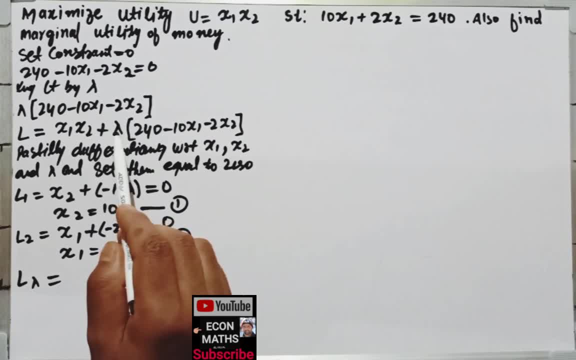 now, here the derivative of lambda is 1, so we will get 240 minus 10, x1 minus 2, x2, that is equal to 0. now solving, and let this be equation third, now to get the value of x1 and x2, we will, we will divide equation 2 by 1, so dividing 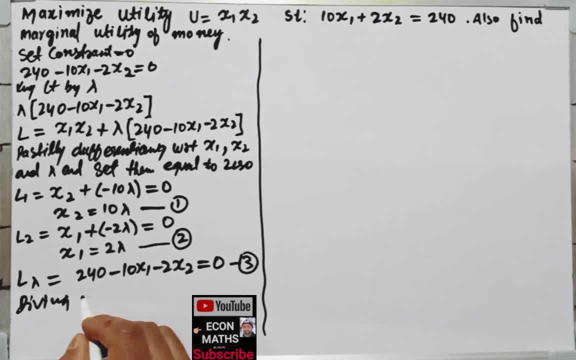 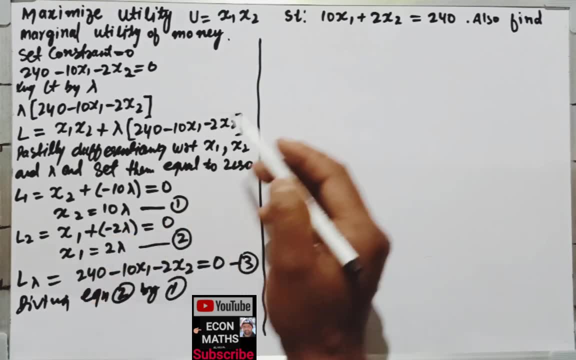 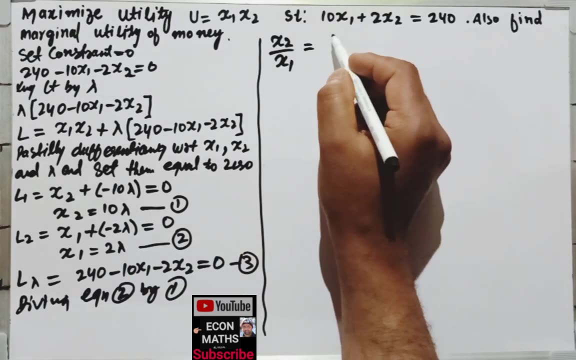 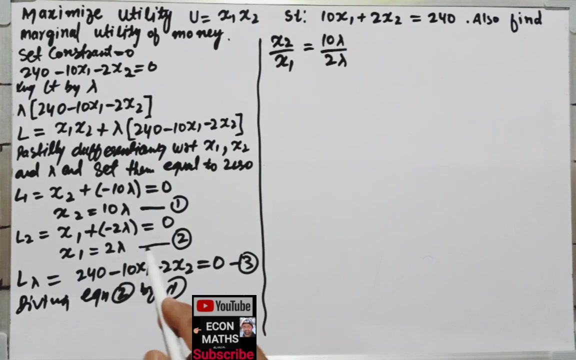 dividing equation, equation 2 by 1, so this will become x2 divided by x1, so this will become x2 over x1, and on our hs this will become 10 lambda over 2 lambda. here it is 10 lambda over 2 lambda. now, further solving this implies: 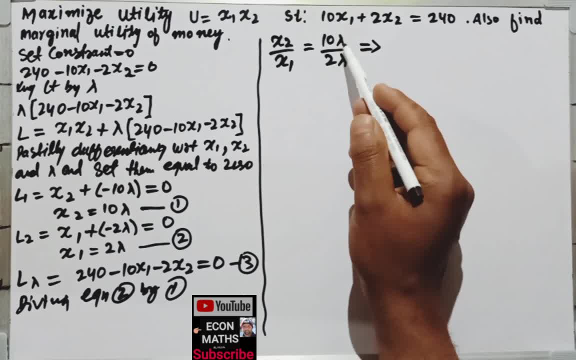 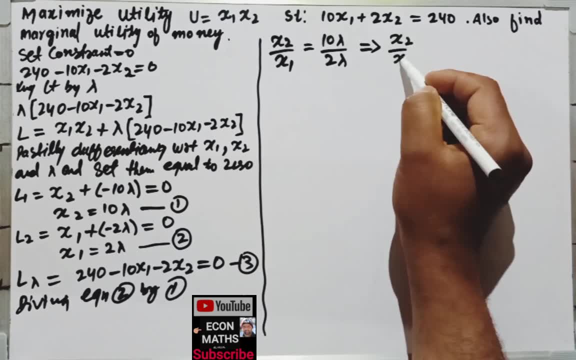 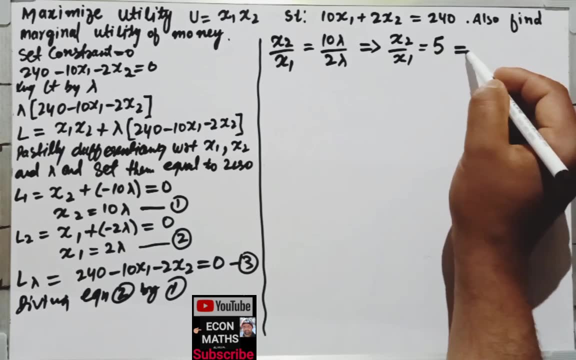 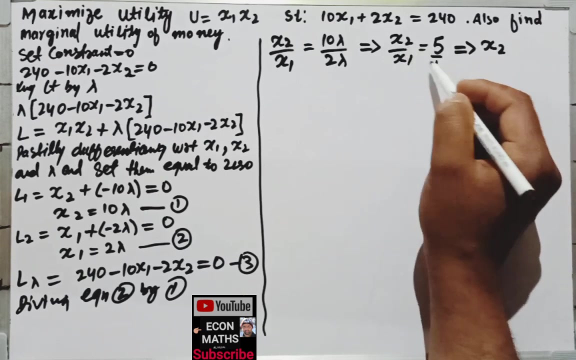 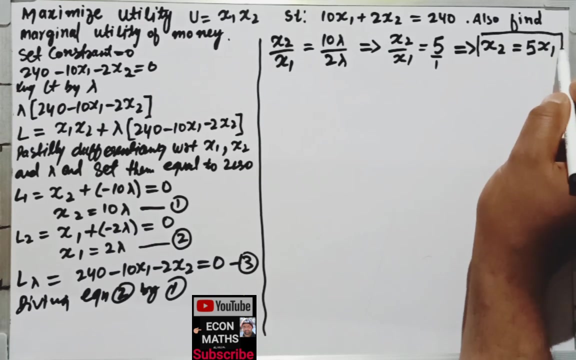 this will become lambda, and lambda will cancel each other, and two ones are two, fives are 10, so this will become x2 over x1 is equal to 5 or or x2 world. that now we solve x2 linear. of course we solve at. 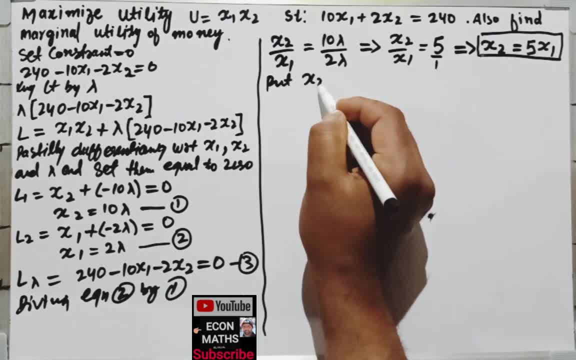 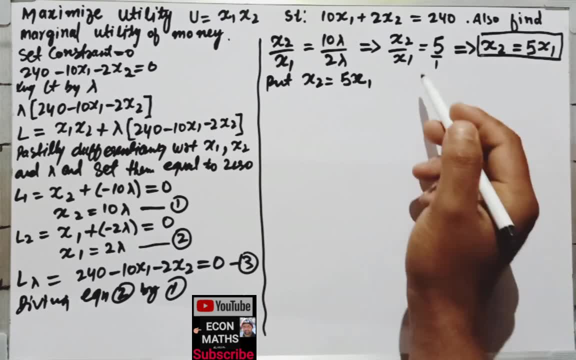 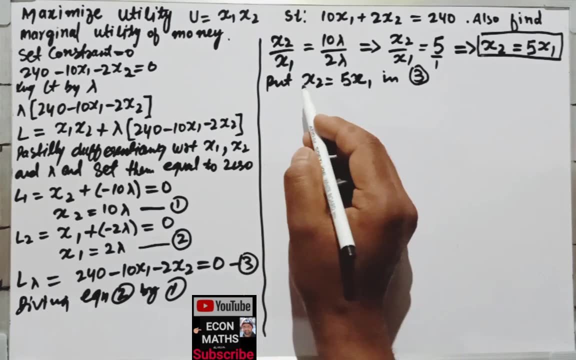 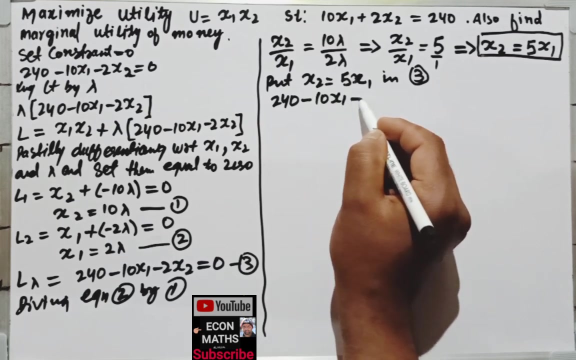 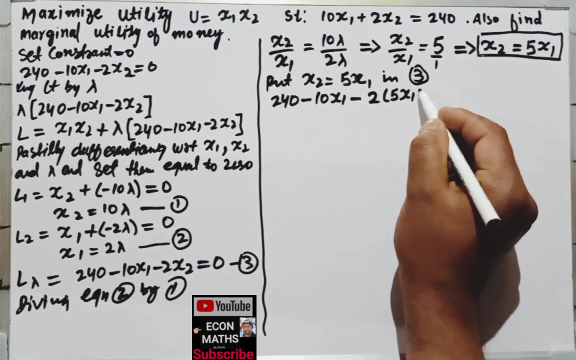 now we will solve x1 and x2 into one. so once again put the new solution in a entertainer. we move it around. so we just do x2 external with x1 third. so this will become 240 minus 10, x 1 minus 2. now the value of x 2 is 5 x 5 x 1 and set it. 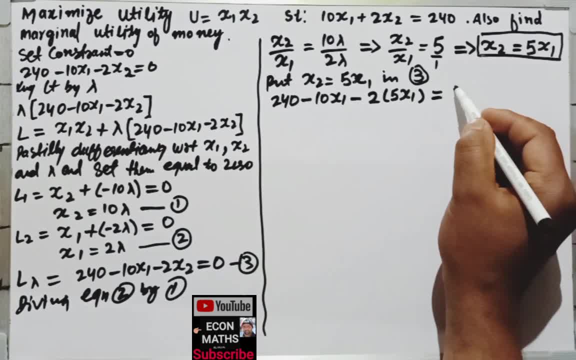 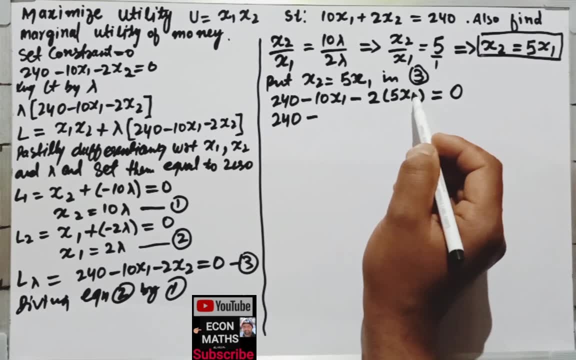 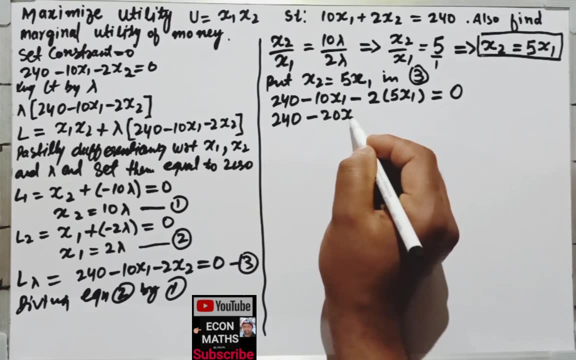 equal to 0, as it is in the equation. third: now this is 240 minus this is two fives are 10 x 1 and here also it is 10 x 1. now minus 10 x 1, and minus 10 x 1 is minus 20 x 1 is equal to 0. 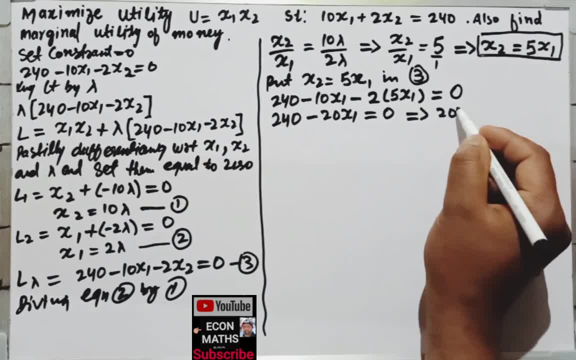 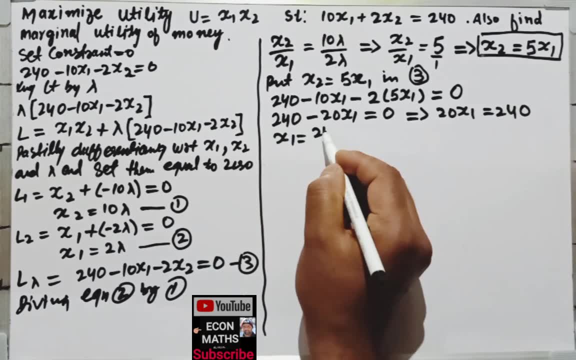 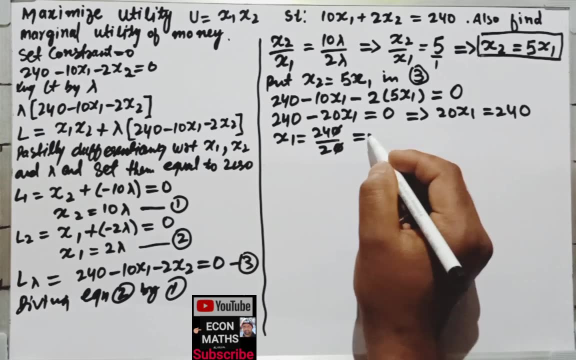 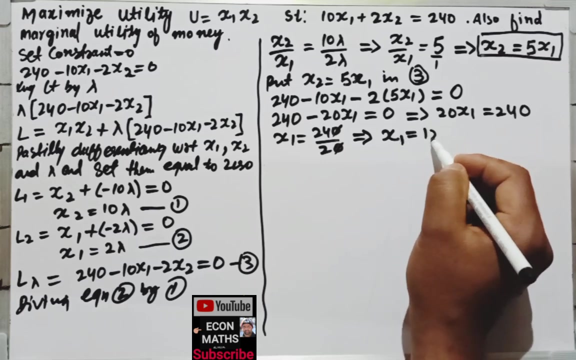 implies 20, x 1 is equal to 240, or x 1 is equal to 240 over 20. so this is uh now further solving. this implies the value of x is 2, 1, 0, 2 tools are, so the value of x 1 is 12. 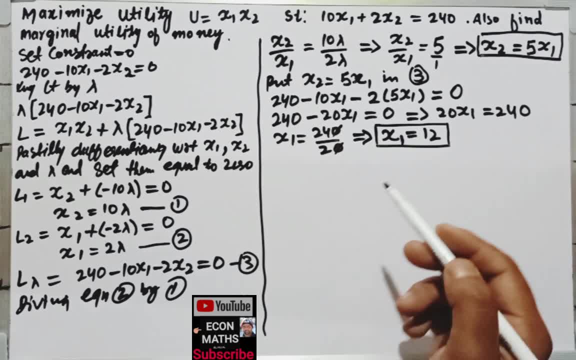 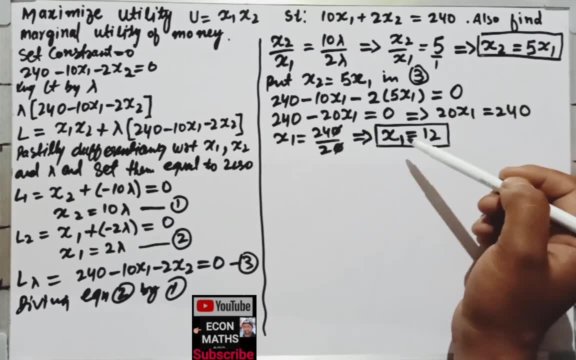 now we will put the value of x 1 in equation, or i will put the value of this x 1 in this. let this be equation 4. so i will write this as equation 4. now, put x 1 is equal to 12 in equation. 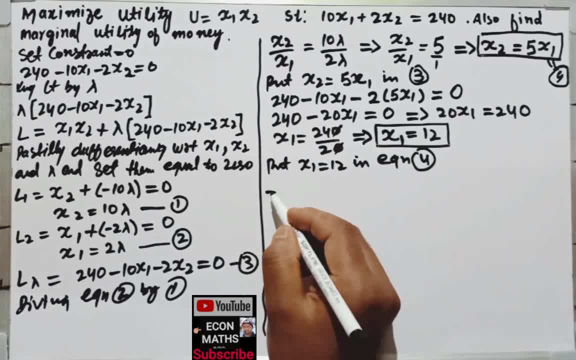 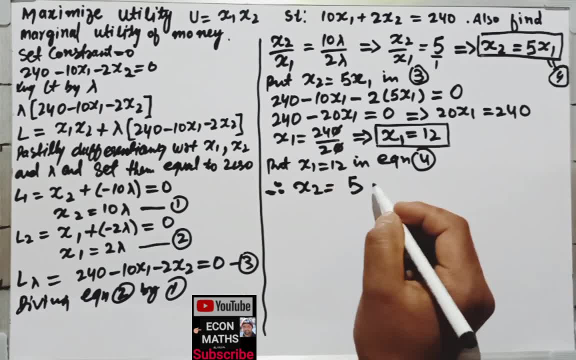 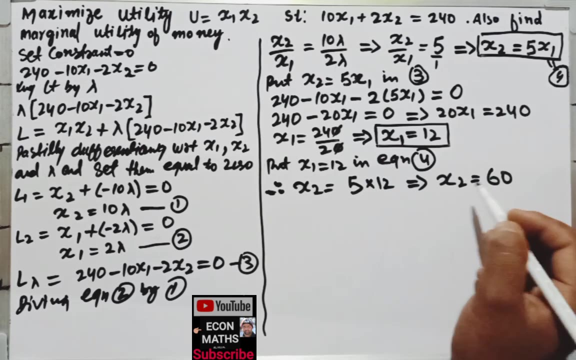 equation 4 now. therefore, therefore, x 2 is equal to 5 times now. the value of x 1 is 12. implies: implies the value of x 2 is x 2 is 5. tools are 60.. now we got the value of x 1 and x 2. 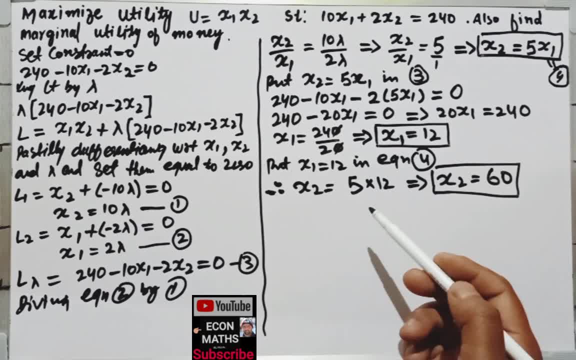 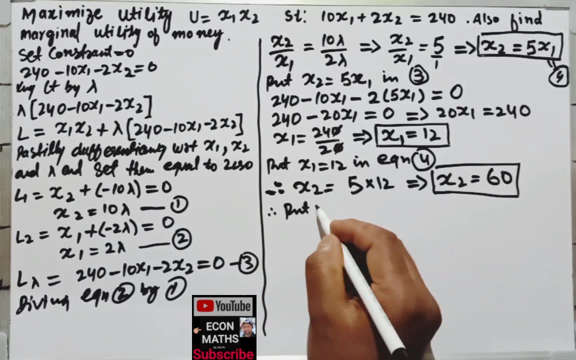 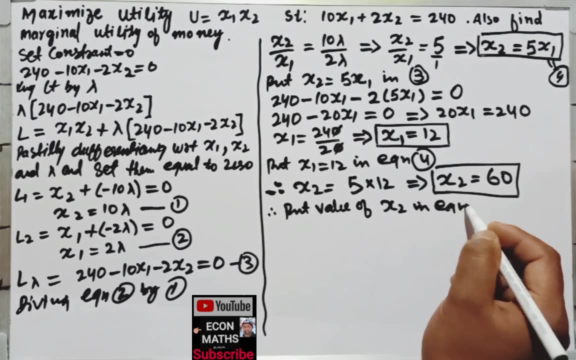 now we will find the value of lambda. now, therefore, to find the value of lambda, we will put the values of x1 and x2 in either equation first or second. so therefore, put value of x2 in equation, equation first. now the equation first is now: x2 is x2 is given that is 60 is equal to 10 times lambda implies lambda. 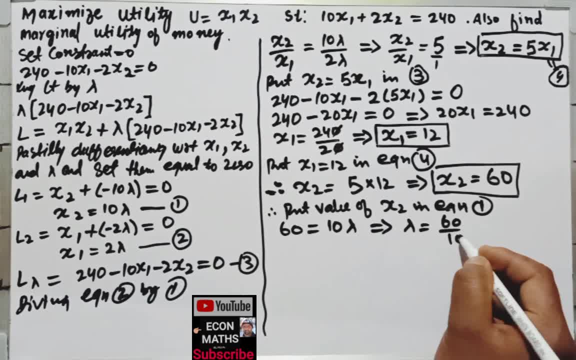 is equal to 60. our 10, that means lambda is equal to 6. now the optimal bundle is: X 1 is equal to 12, X 2 is 60 and lambda 60. is 6. now the value of lambda tells us if there is incremental one unit change in the constraint. 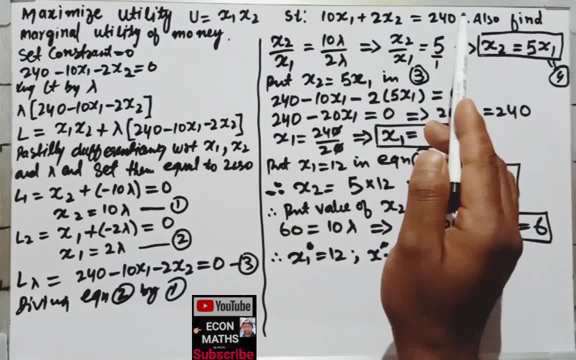 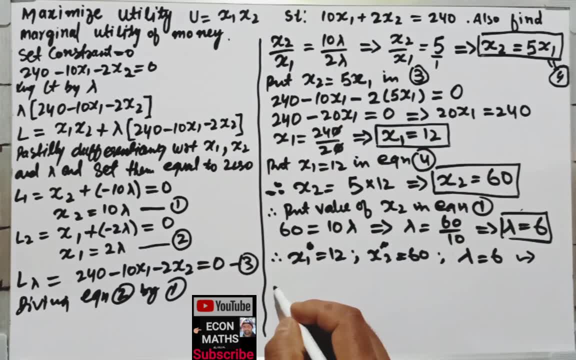 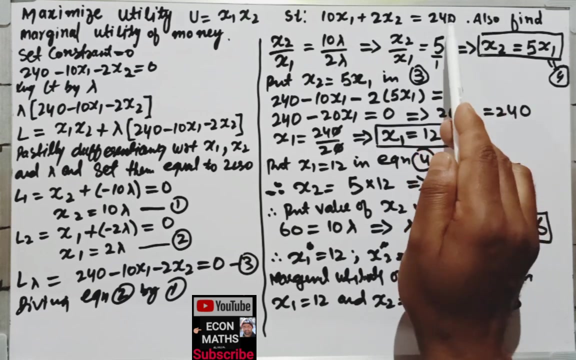 constant of this constraint. the constant of this constraint, the utility will change by six units. that means the marginal utility, marginal utility, utility of money, when, when x 1 is 12 and x 2 is 60 is six is six. that means, if the, if the budget changes by one, 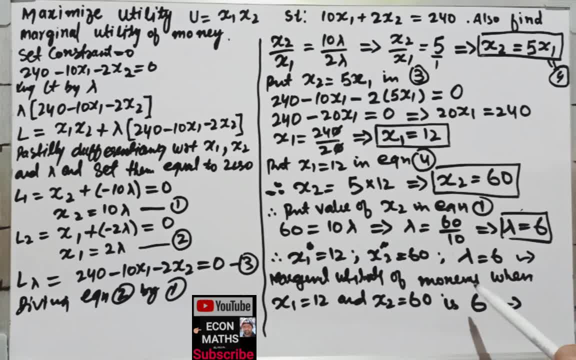 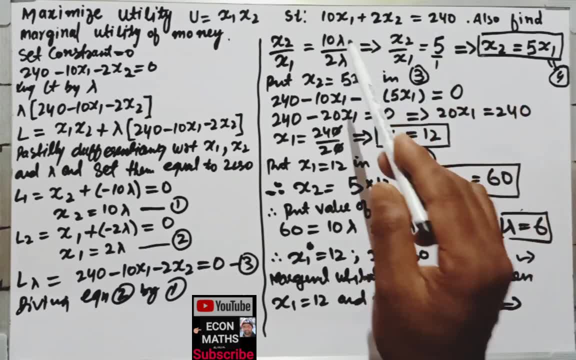 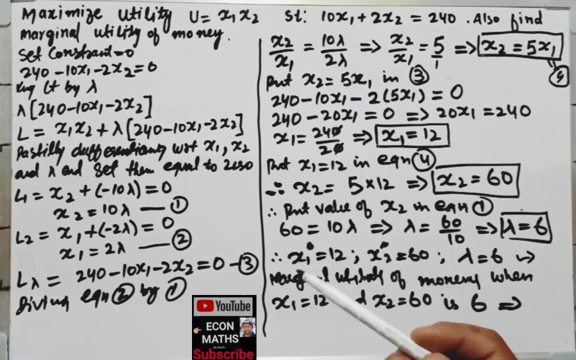 unit, there will be six units change in the utility function or if the budget increases by one unit, utility will increase by seconds units. so this was all about maximizing utility functions. i hope you enjoy the video. if you, if you really enjoyed the video, please subscribe and share.